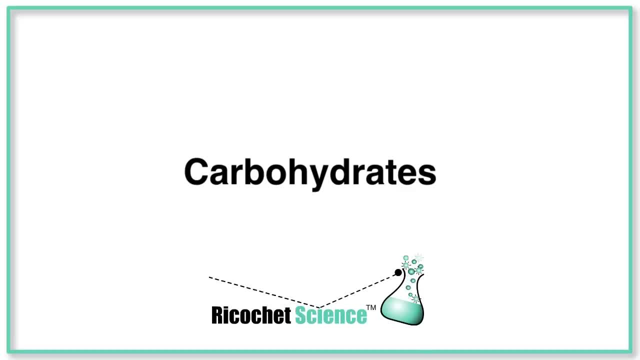 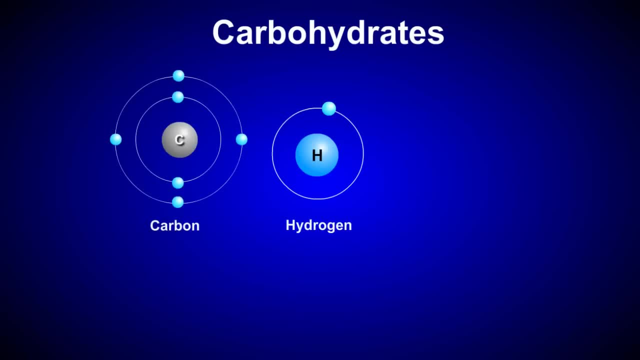 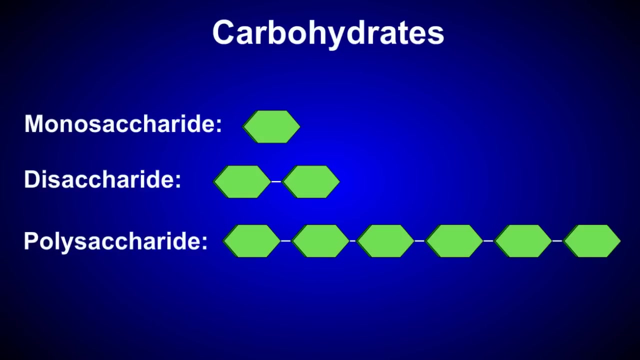 Carbohydrates are biomolecules that are composed of carbon hydrogen and oxygen atoms in the ratio of 1 to 2 to 1.. We can represent the proportion of these elements within carbohydrate molecules with the formula C-H2O. Most carbohydrates are characterized as either monosaccharides, disaccharides or polysaccharides. 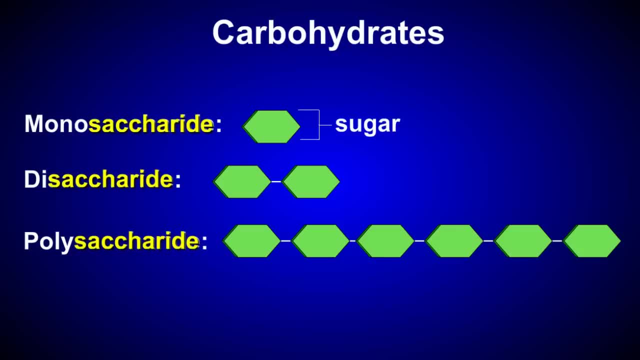 The term saccharide is just another word for sugar. The prefixes mono-, di- and poly- refer to the number of sugars in the molecule. Mono- means one, so a monosaccharide is a carbohydrate made of one unit of sugar. 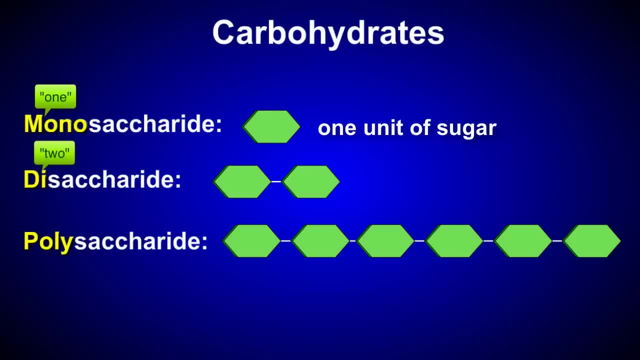 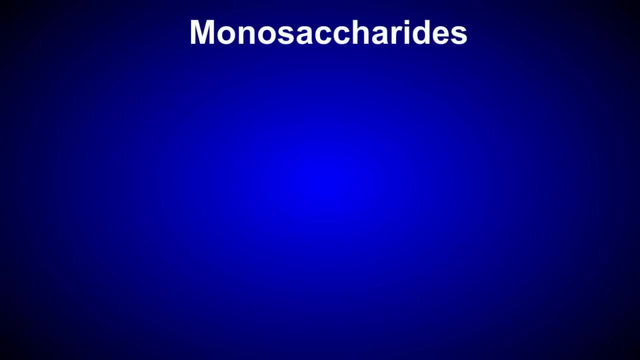 The prefix di- means two, So a disaccharide is a carbohydrate made of two units of sugar, And poly- means many, so a polysaccharide is made of many sugar units bonded together. Let's talk about monosaccharides first. 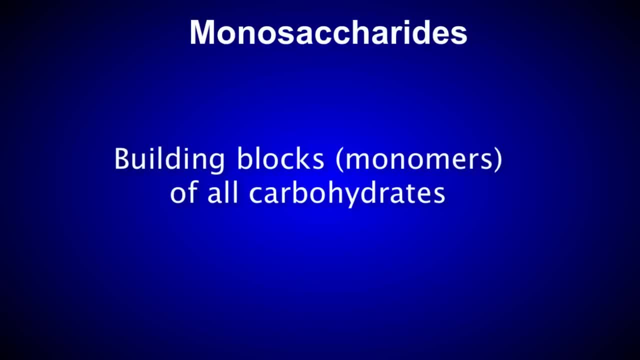 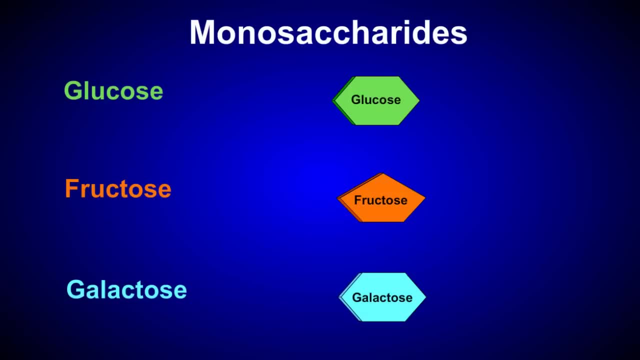 Monosaccharides are the building blocks, or monomers, of all carbohydrates. Common monosaccharides include glucose, fructose and galactose. Glucose is by far the most abundant monosaccharide. It's water-soluble, easily transported through an organism and is the energy source for. 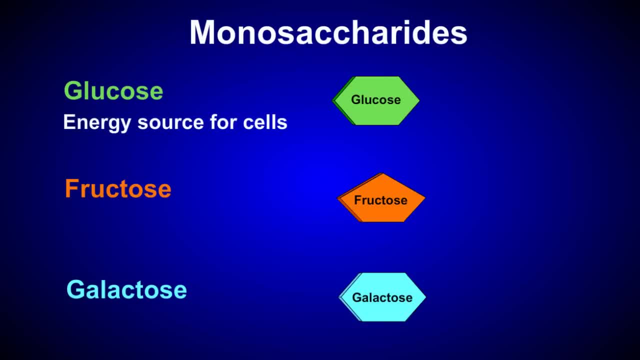 cellular respiration and the production of ATP. Fructose is the primary monosaccharide found in fruits and plants, and galactose is the primary monosaccharide found in milk. All of these monosaccharides are six carbon sugars with the chemical formula C6H12O6. 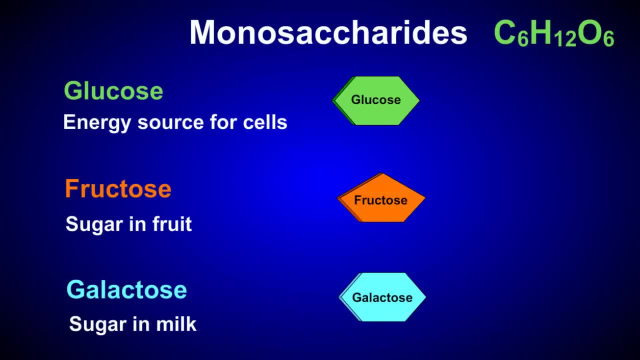 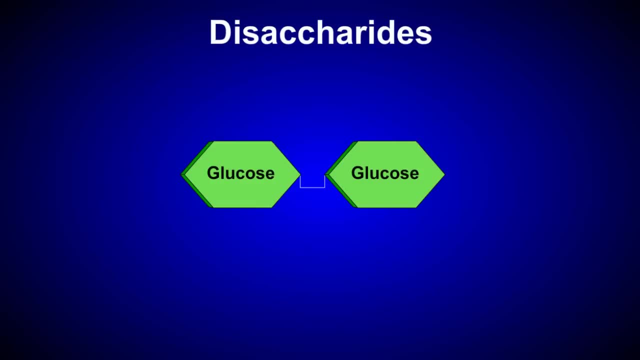 They can be depicted chemically as either straight chains or straight lines. Disaccharides are formed when monosaccharides are joined together through dehydration reactions, forming what are called glycosidic linkages. Common disaccharides include maltose, which is made up of two glucose molecules: sucrose. 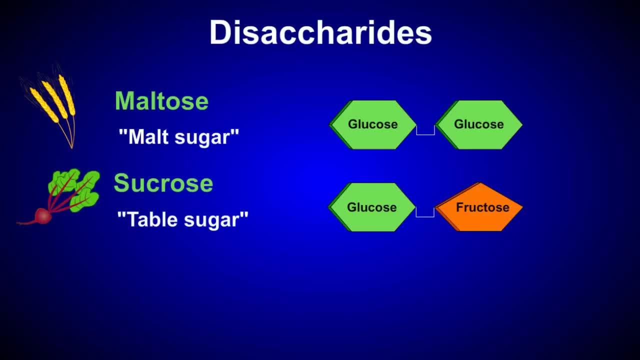 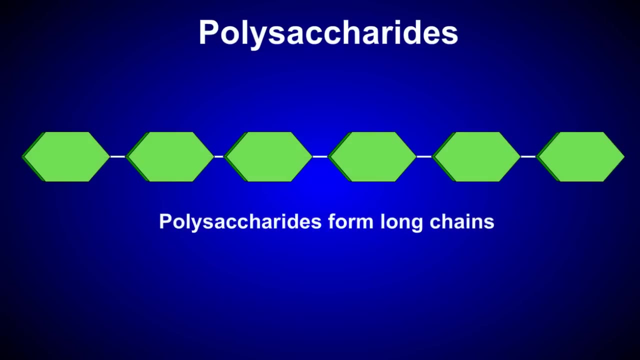 also known as table sugar, which is made up of glucose and fructose and lactose, or milk sugar, which contains glucose and galactose. Polysaccharides are formed when glucose monomers link together to form long chains. These long chains of glucose units are ideal for storing energy.